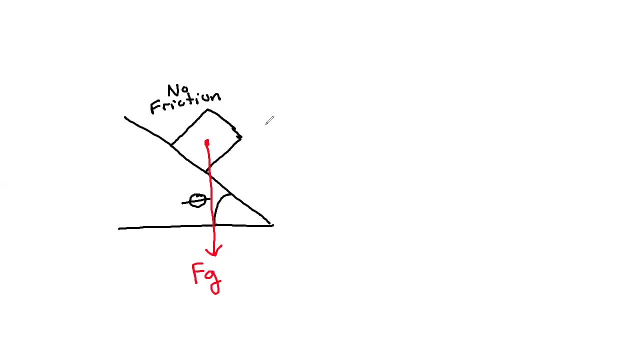 in the way. So what's going to happen is we are going to have a direction of motion. direction of motion that's going to be more like this, way down the incline, And we're going to call that the component of the weight parallel to the incline, FG parallel. And then also, because this box pushes into the surface a little bit- the surface, we know, because Newton's third law says that there's going to be a force that's going to be perpendicular to the surface. 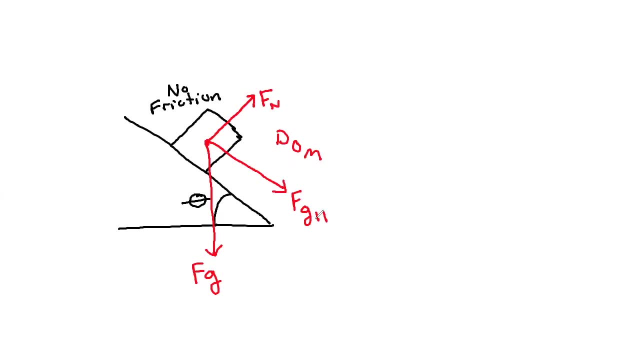 That we call the force of the normal. These three forces, guys, like I said, regardless of whether there's friction or not friction, these forces are always going to be there And we can solve for these in certain ways. FG, we've already learned- is just M times G, where G is the acceleration due to gravity And on the AP level we just call that meters per second squared. Somewhere else you might see it referred to as 9.8.. But to keep our math simple, I'm going to call it M times G. 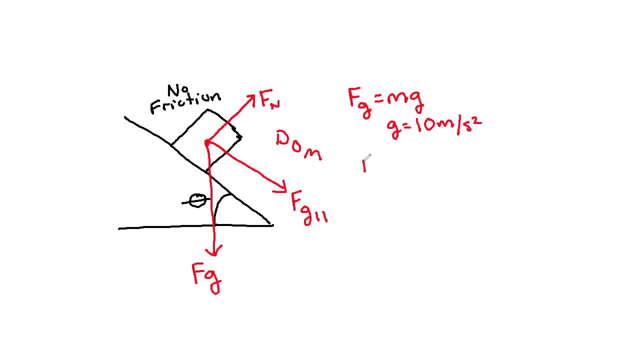 10 meters per second squared. Now we know that FG- parallel and F- normal are components of the weight, So MG must be there, They have to have some sort of weight associated with them. Okay, but now because that inclines there, we have to factor in the theta. And the way we do so is when we're going down the incline we use the sine of theta, And so 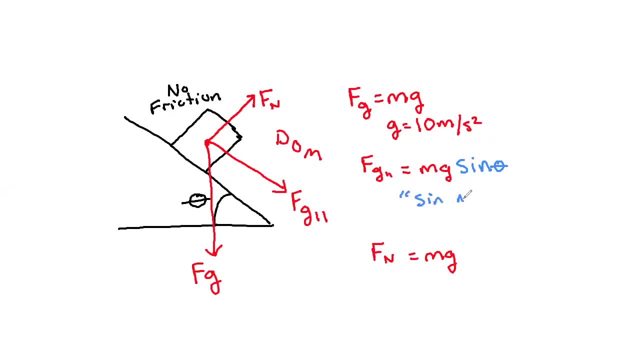 to remember this. I remember sine makes it slide, All right, and that's going to be the force that is going to make that slide down the incline. Now, the force of the normal is going to be the cosine of theta And we remember that. cos keeps it close? 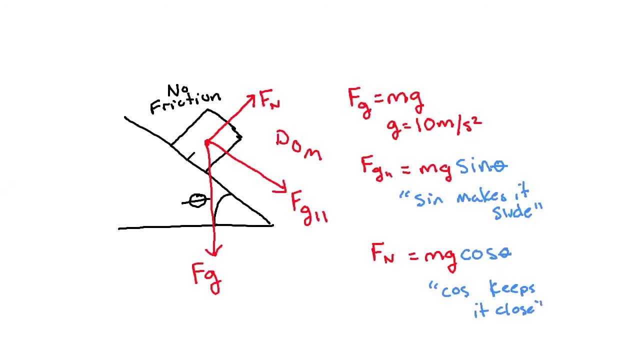 All right, this is the force that's going to keep it near the incline right here. So these guys are the only forces and the only components that are going to be acting on a box with no friction. Okay, so now we can look at Newton's laws And we can say that excellent A, we know A- equals F net over M And the F net is only going to be associated with the delta. 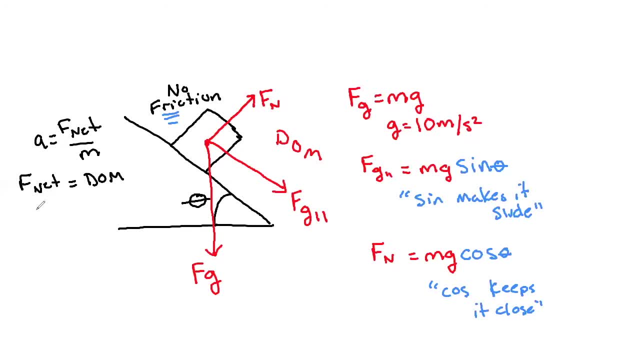 Direction of motion. So we don't have to worry about Fn in this case, because it's not in the dom, It's not in the direction of motion. So I'm only going to look at forces that are associated with the direction of motion, And the only thing in the direction of motion is Fg, parallel. 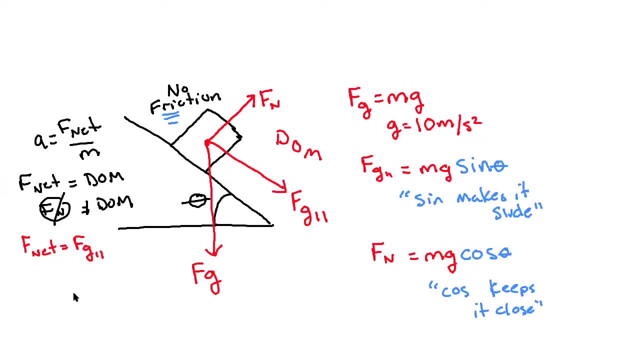 So now, when I want to solve for A, I see that A is equal to Fg parallel Over the total mass of the system And Fg parallel is Mg. Sine makes it slide- Theta divided by M. Okay, and look at this. This is wonderful Boom. So now we have an expression that we can use for an incline And we could say that A is going to be equal to G sine theta. 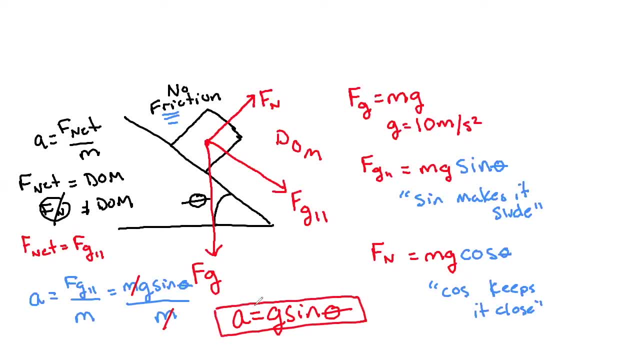 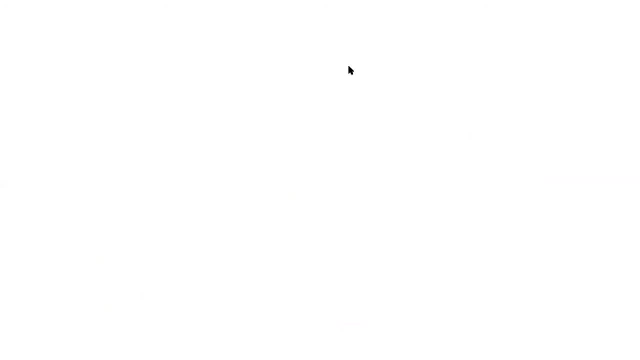 All right now let's take a look at an example of this using some numbers. If I look at an incline here, Let's give this incline an angle of, say, 30 degrees. Don't forget, guys, degree sine is a unit. 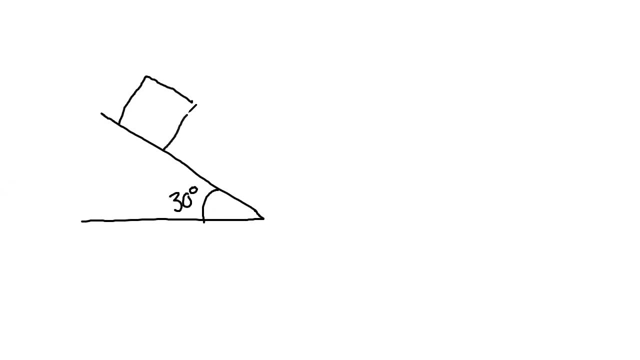 And then we'll have a box M1. And we'll say that M1 has a mass of 20 kilograms. Okay, so, awesome sauce. Let's take a look at all those three forces I said we have to have on there. We have to have Fg, We have to have Fg parallel. 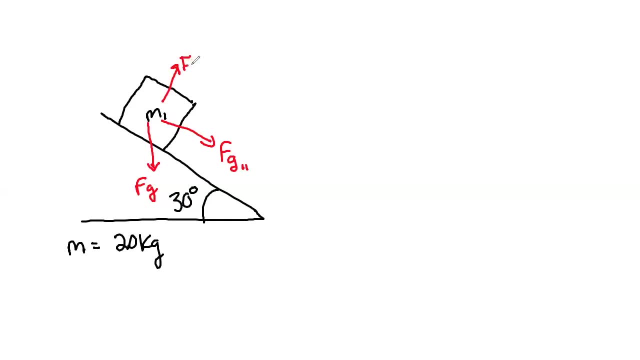 We have to have the force of the normal. These three will always be there, And when there's no friction, that's going to be it. So now we jump in and we say that A equals F net in the dom, All right, And guys, this will keep us. I'll remind you what the direction of motion is. Don't forget, the dom is just going to be down the incline Right, So we don't have to worry about the force of the normal in this case, because it's not in the dom.